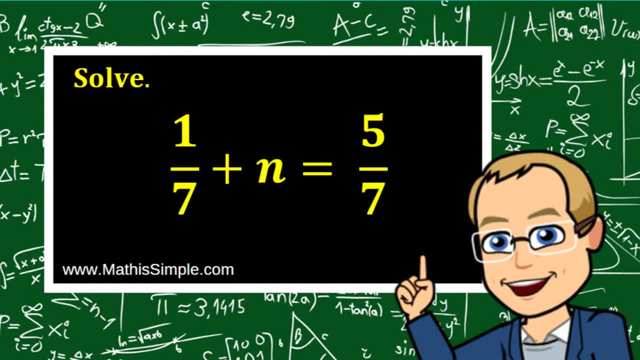 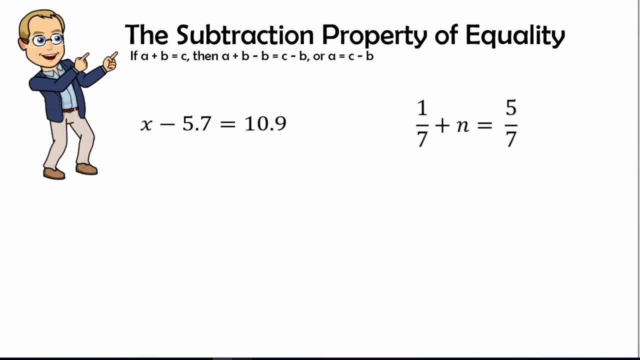 In part two of learning about one-step equations and the subtraction property of equality, we would like to look at equations that have decimals and fractions involved in them, And in this first equation we see that we have x minus 5, and 7 tenths is equal to 10 and 9 tenths, So we 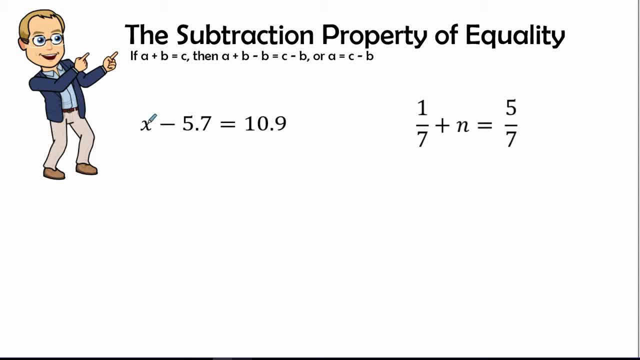 look at our variable here, x, and we see what's attached to it. And we see that the 5 and 7 tenths is attached to it. How is it attached? It's attached by subtraction, So the inverse of subtraction is addition. So we are going to add 5 and 7 tenths to both sides of the equation. 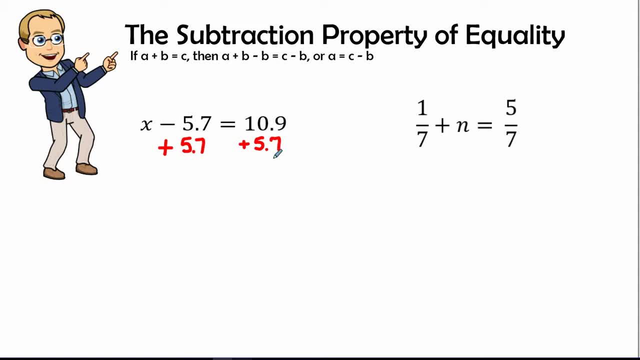 When we're dealing with decimals, we're going to try to make sure to keep our decimals in line with each other. So I'm going to go ahead and erase this a little bit and rewrite it for you, And so we have 5,, which is in the ones place, and 7,, which is in the tenths place, And so our 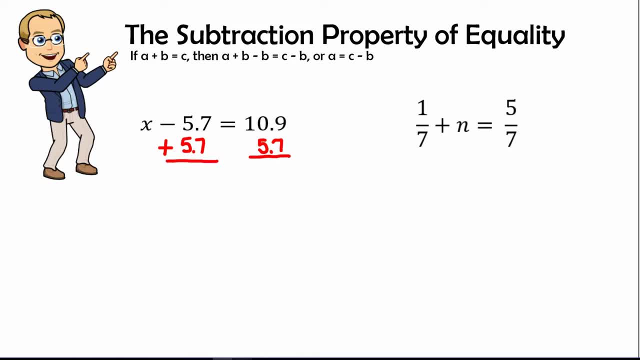 decimals are in line with each other. Now we look at a negative 5 and 7 tenths plus 5 and 7 tenths, and that is the inverses of each other, And so that is going to equal 0.. So we're going to bring 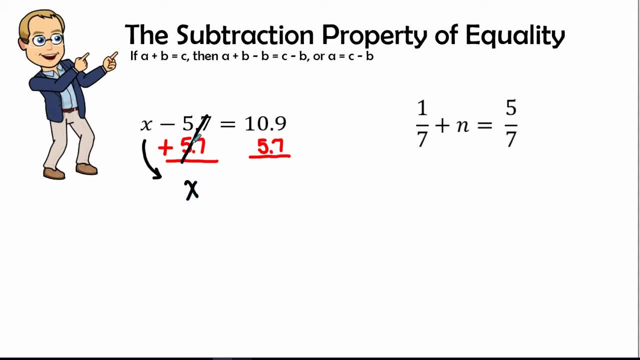 down our variable x and it'd be x plus 0, but that 0 would drop off. And then we're going to add 5 and 7 tenths to 10 and 9 tenths, So 9 plus 7 is 16.. 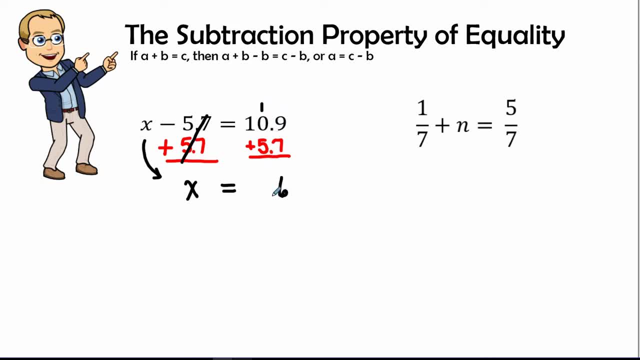 We're going to carry our 1, and we're going to bring our decimal down right in the middle or right in line with each other. 5 plus 0 is 5, plus 1 is 16, or 6, and 16.6 is our answer. 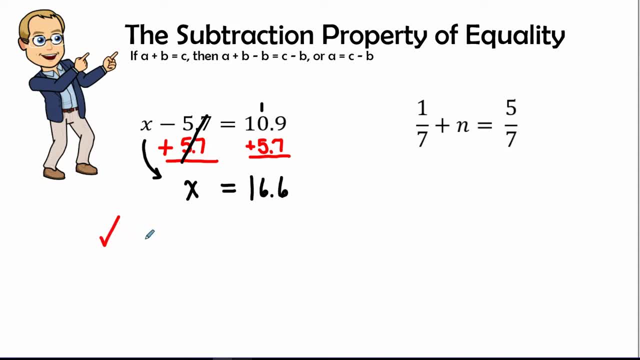 And so then we go ahead and double check our work. We are going to wherever we see our variable. we are going to write 16 and 6 tenths and it's gonna subtract 5 and 7 tenths, and that should equal 10 and 9 tenths. 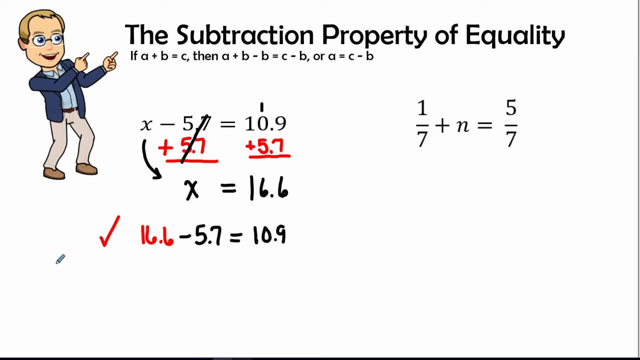 So off to the side, I can go 16 and 6 tenths minus 5 and 7 tenths. I'm going to go ahead and do that. I'm going to go to And borrow, or let's see we are going to bring that to a 5, add a 1 whole point. so that's a tenths, 10 tenths. 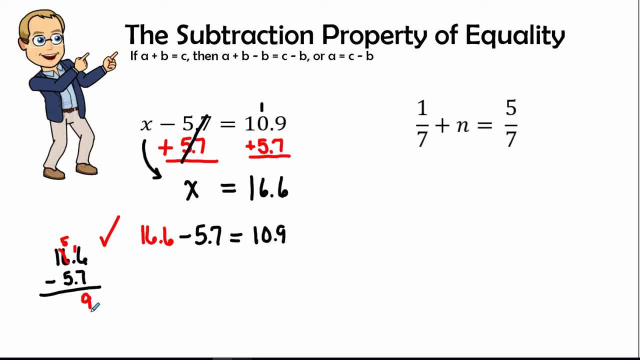 So 16 minus 7 is 9,, 5 minus 5 is 0, and 1 minus 0 is 10.9.. So we know that 10.9 here is equal to both sides. Therefore our answer is correct. 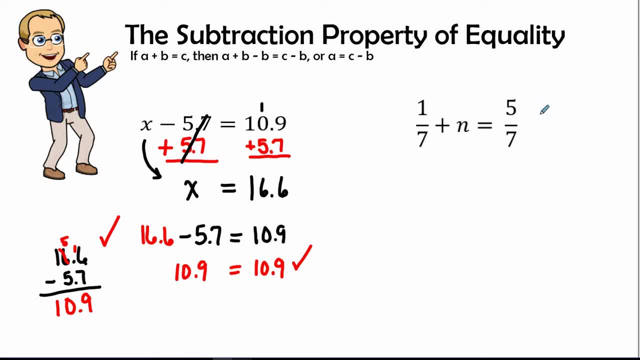 Now, moving on to the second problem, or the second equation, this equation has fractions in it. So we look at the equation and we see 1 seventh plus the variable n equals 5 sevenths. So this 1 seventh, it doesn't have anything in front of it, but we do know. if it doesn't have anything assigned in front of it, it is positive. 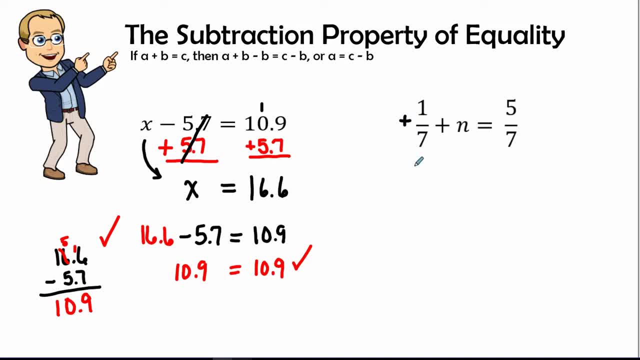 So that helps us out What's attached to the variable n? It's a positive 1 seventh. so the inverse of a positive 1 seventh is a negative 1 seventh And we are going to subtract 1 seventh or add 1 negative 1 seventh to both sides. 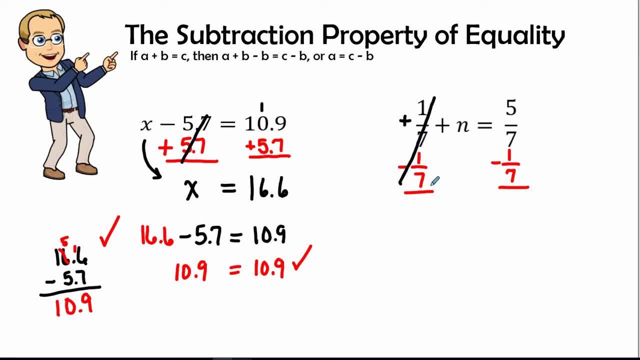 Now we see that these are inverses of each other. as always, it equals 0,, leaving a positive n by itself. Here we have our equal signs in line with each other, And then we can also- Let's do this problem horizontally. 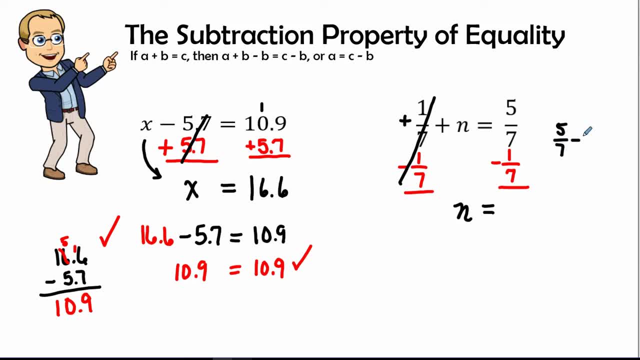 So I could say 5 sevenths minus 1 seventh, and I have like denominators, so I can keep the denominator the same, and 5 minus 1 is 4.. So the variable n is equal to 4 sevenths. 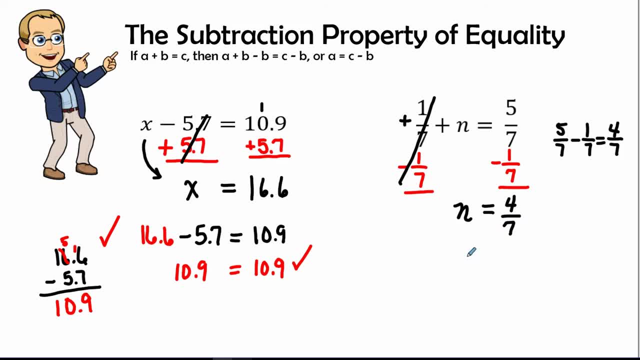 Let's go ahead and plug that into the equation. So I have Remember, I have the 4 sevenths for the variable And I'm going to add 1 seventh, and the 1 seventh equals 5 sevenths. Therefore, 1 plus 4 is 5..